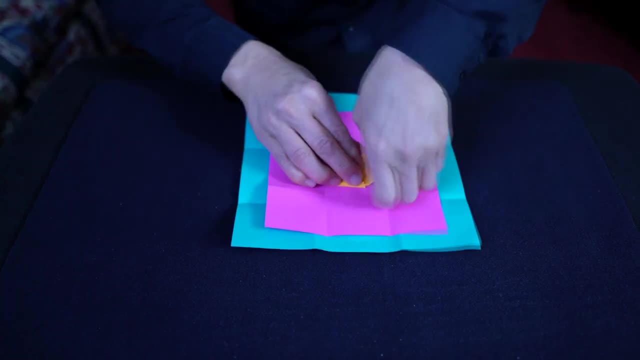 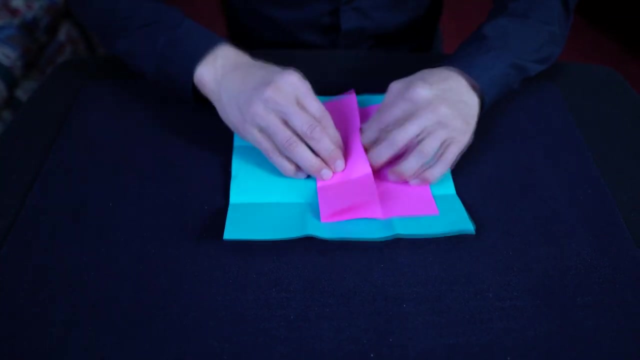 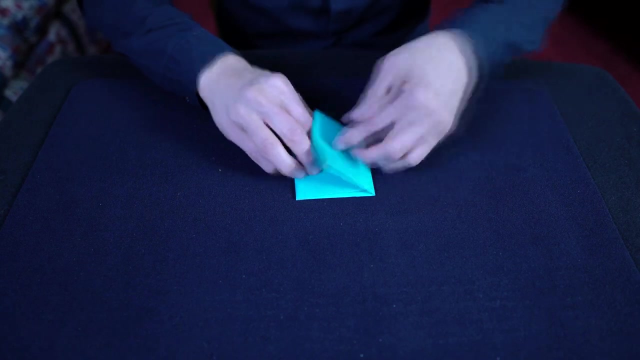 into this piece of paper right here And you'll notice that I have a second piece of paper here. We're going to fold that in And fold the final piece of paper. Now for the magic. Everything should be secure, but if I snap my finger, let's see if some. 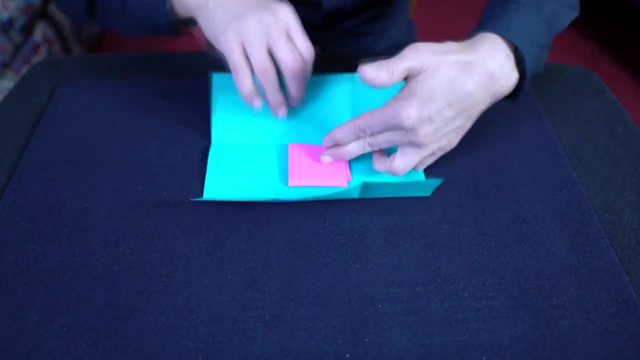 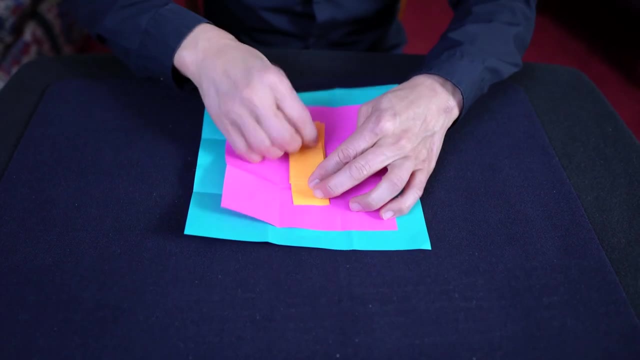 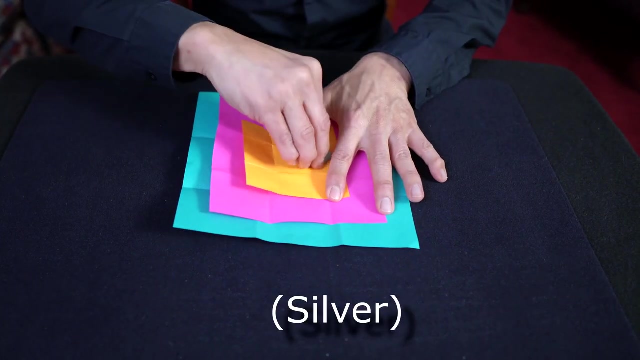 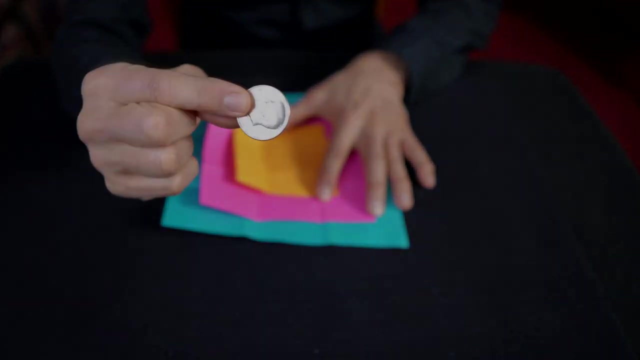 magic occurred. We're going to unfold the paper. Unfold this paper And we have one more paper to go. But look, we now have a silver coin, A Kennedy Half KA. How's that for a magic exchange rate? 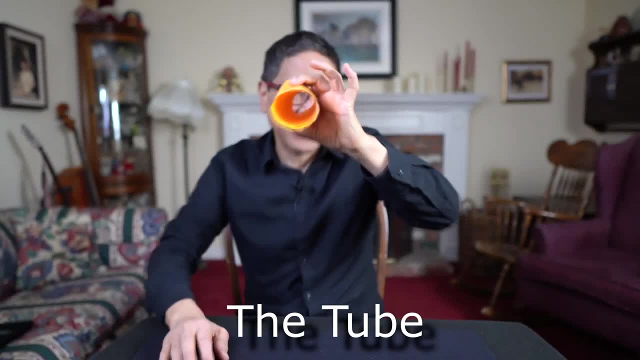 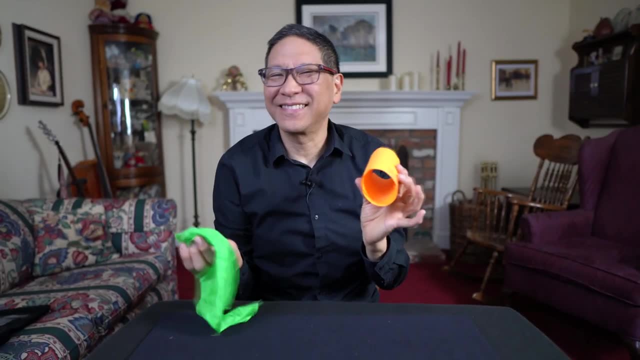 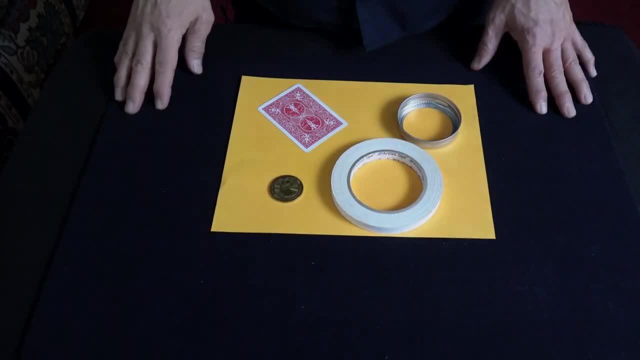 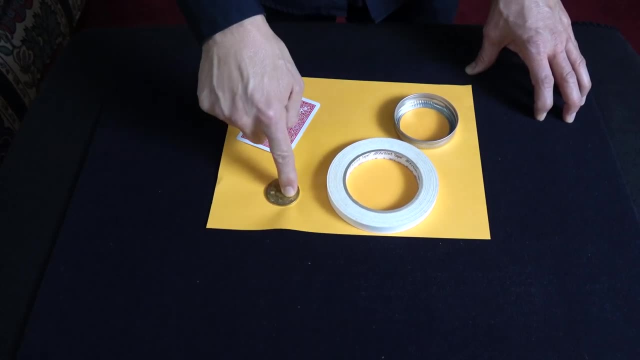 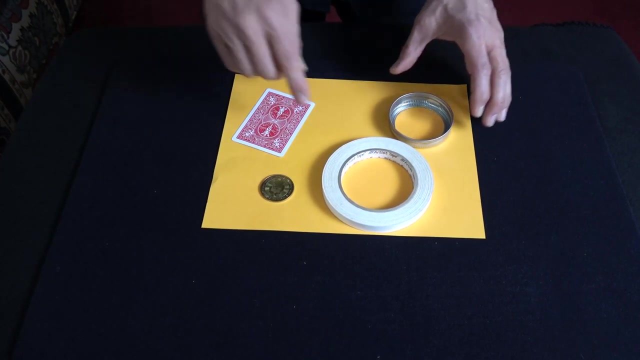 0. 0. 0. 0. 0.. you need a card, you're gonna need a coin- preferably the bigger the better for a more effective vanish- and you're gonna need a piece of paper- actually gonna need two sheets of paper, and I'll explain why. now, what I have here is a 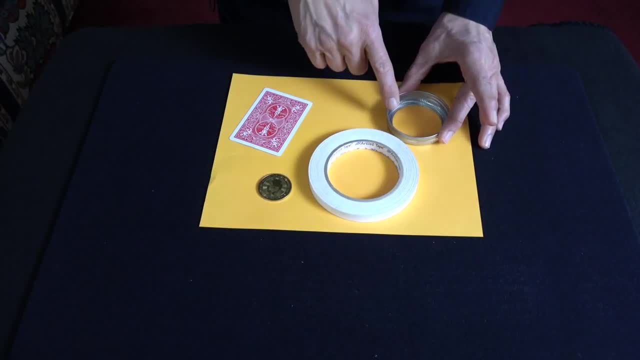 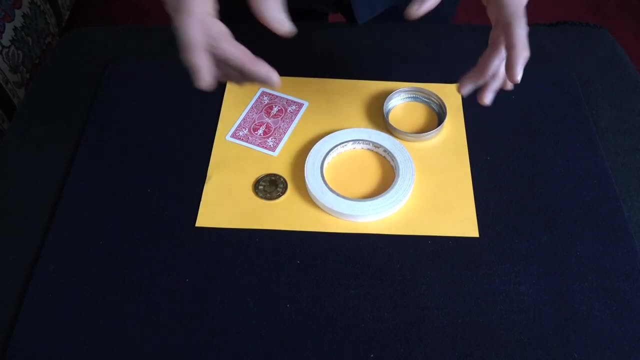 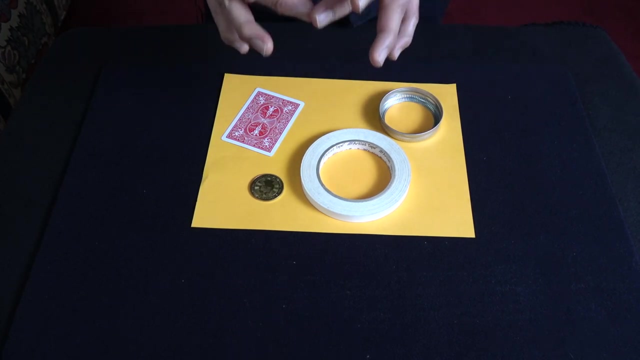 seemingly innocent roll of tape- and this is the top of a mason jar here for making jams, canning jams. I guess what I've done is I wanted to perform this trick without buying anything. normally what I would do is just go to the 99-cent store and buy a bunch of bracelets, because those work great. but I 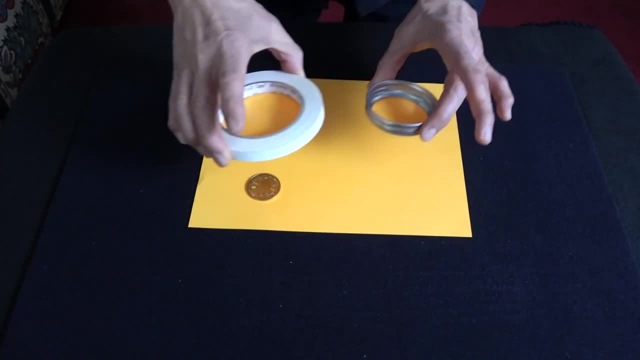 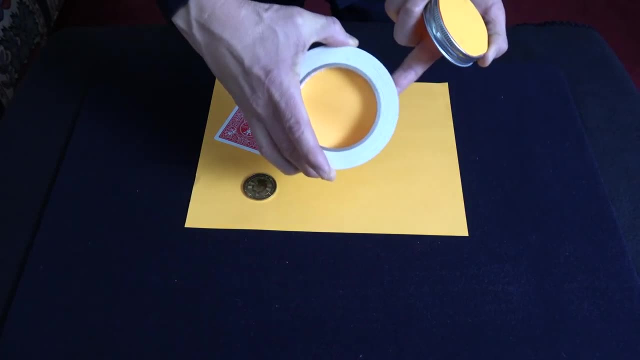 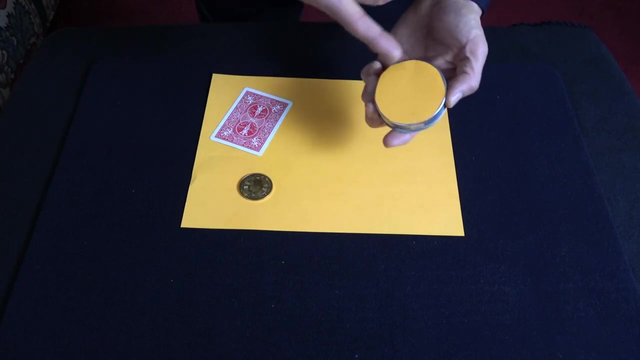 found this roll of tape, I found this mason jar ring, and what I've done is I've taken a piece of matching paper here and cut out a circle to completely cover the openings here, and that's the secret. so once you have your other piece of paper cut out that matches the one that you're performing on, you're ready. 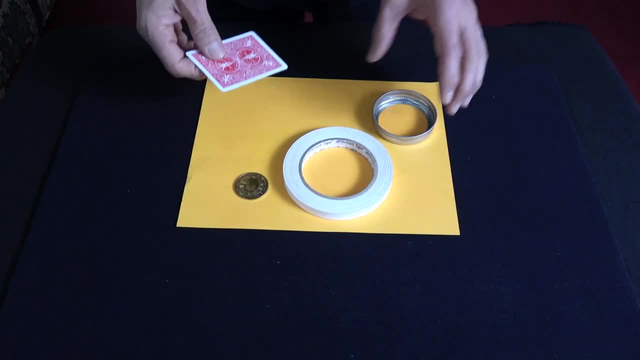 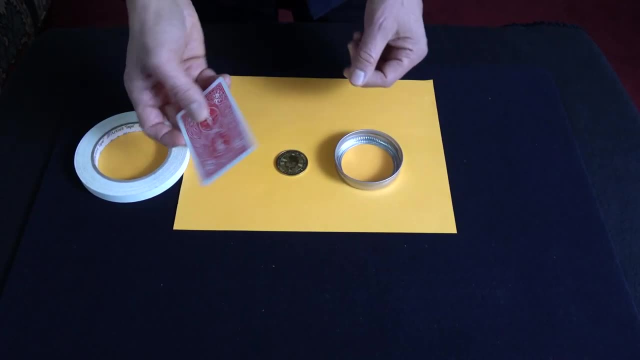 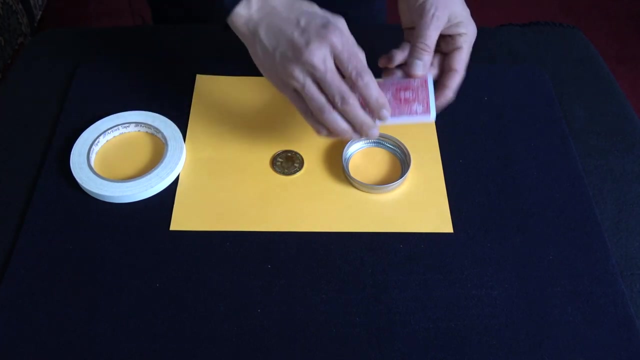 to go, and doesn't that look great? they look completely natural. so what you're gonna do here, we'll use the mason jar. don't do this in performance, but just for explanation purposes. here you have your gimmicked ring, which is the mason ring, here a jar ring, and you have your card, you cover and then you move it over. 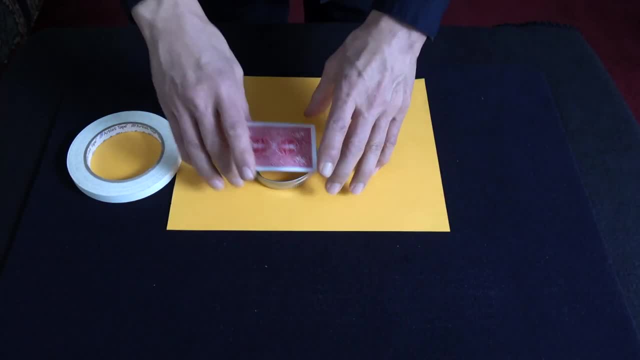 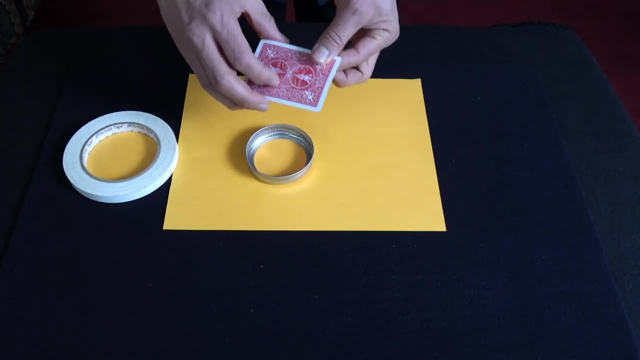 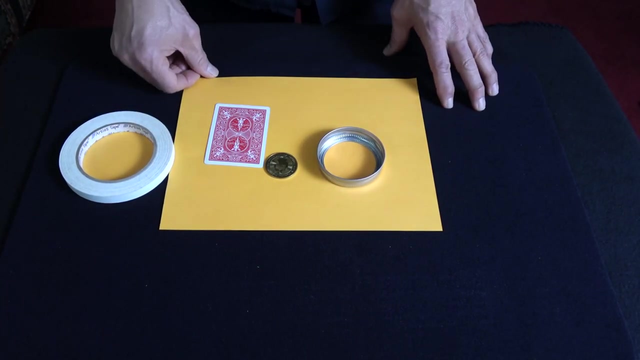 place it over the coin, you snap your finger and the coin appears to vanish, but of course it's just underneath the material here. now you take your card, place it on top, snap the finger and move it over and the coin disappears, returns, and that's the explanation for the vanishing coin. 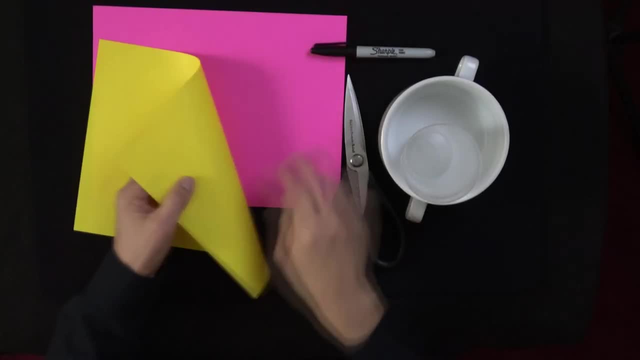 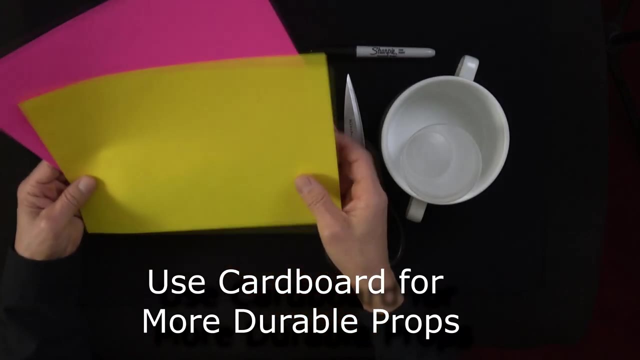 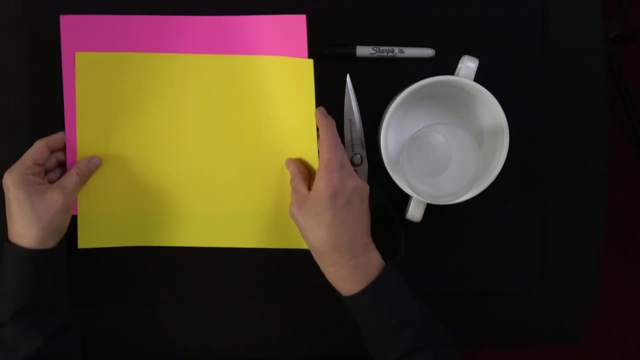 here's what you'll need for the trick: you'll need two sheets of paper. helps to have different color papers and you can use the same colors for the boomerangs, but you'll probably want to label them, so there's a little bit different about them. for the trick itself, 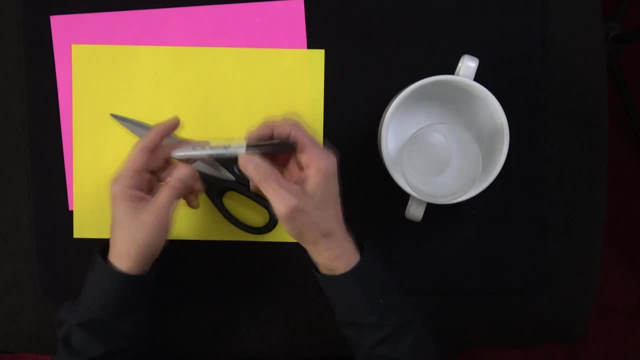 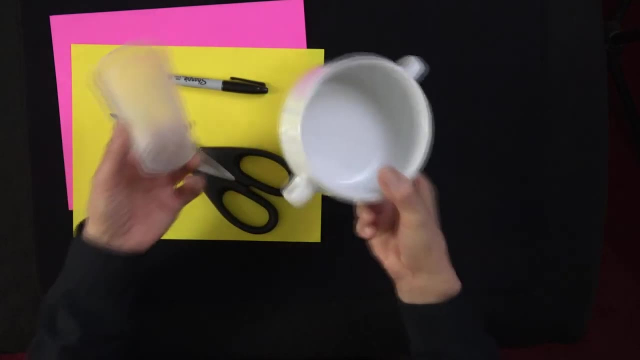 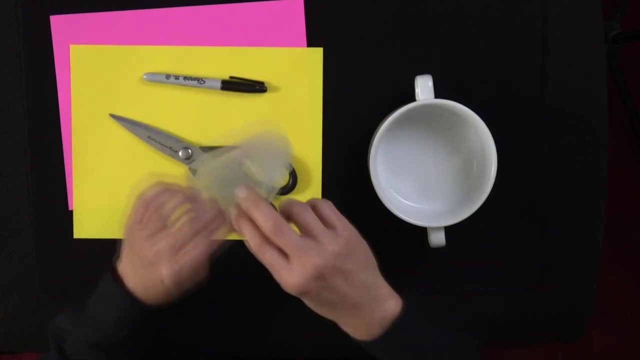 you'll need a pair of scissors, you'll want some type of pen or something to mark with. and what are these? this? what's the cup and the soup mug for? well, this is so. you can actually use the same color paper for the boomerang. so let me show you how to do that. so let's set this. 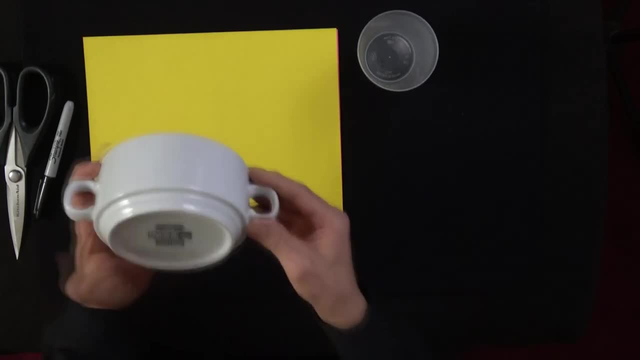 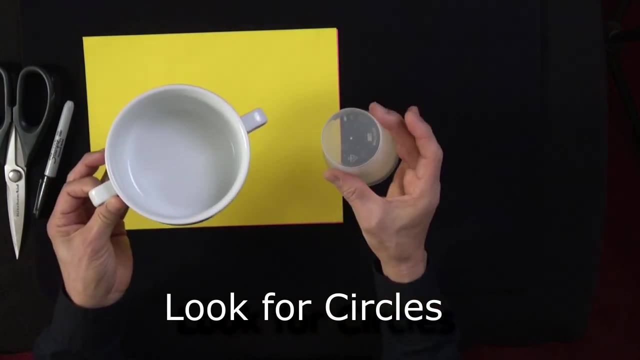 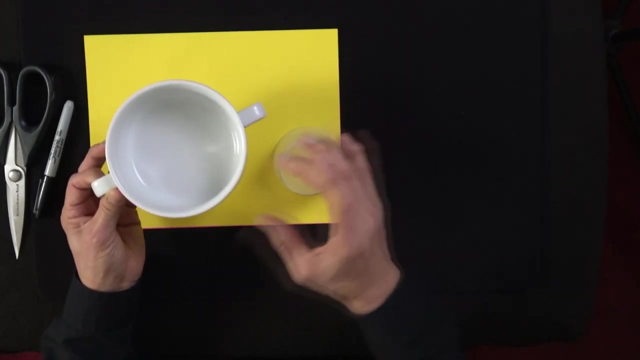 aside for now. take your two sheets of paper, line them up. what you're going to do is take your. you have to go through the house and look for circles with bowls, plates, cups, whatever you have. i've chosen these two because what i want are two different diameters. there's a diameter here and 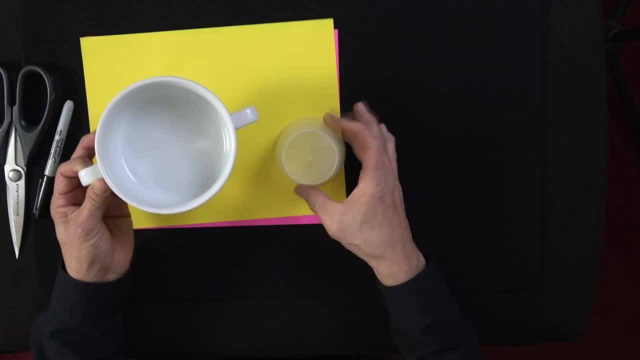 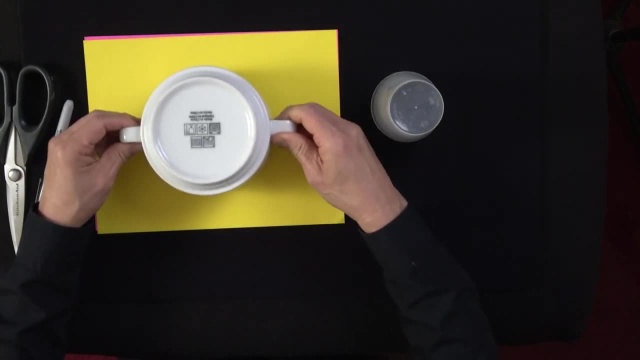 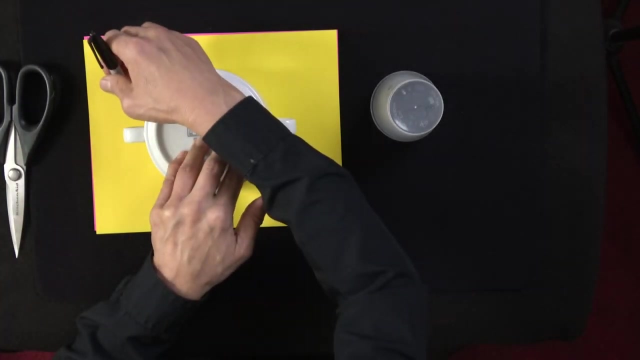 a diameter here, so one: the larger diameter object's going to create the outer diameter. the smaller one will create the inside diameter. so let me show you how that works. i'm going to take this, place it down, i'm going to trace along the edge. all i need is a semicircle, so let's just do. 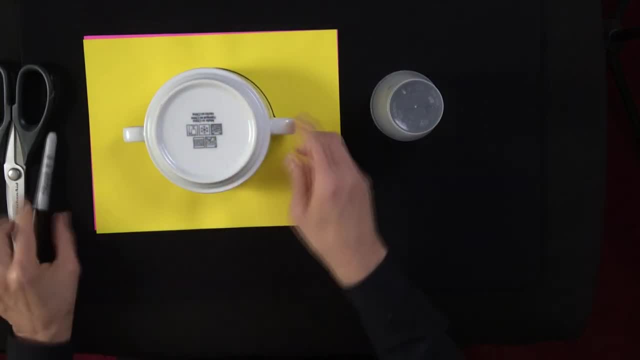 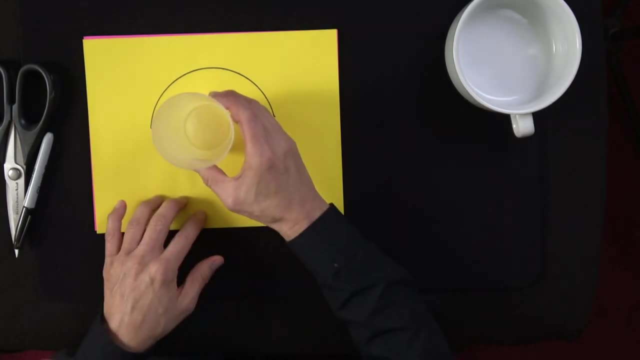 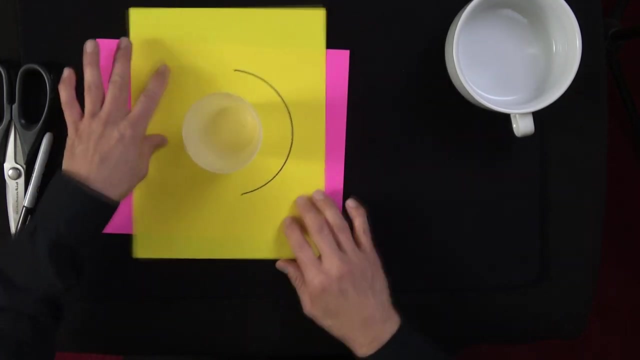 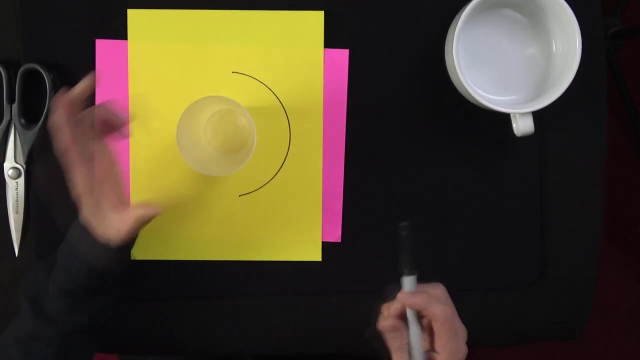 that, and i have a semicircle now with this one. i'm going to use this small diameter here to make an inner diameter. now it's important to try and get this lined up, so. so this is at the center here of the outer diameter. so i'm just going to estimate here and let's draw an inner diameter. 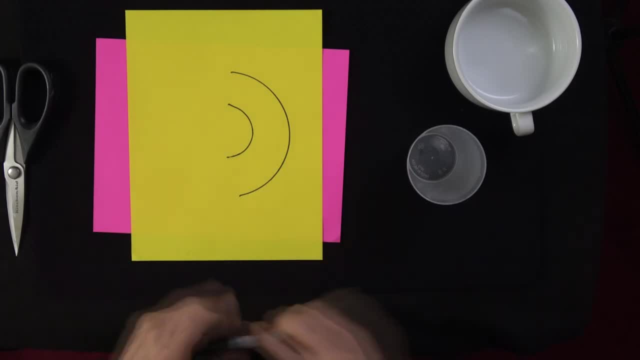 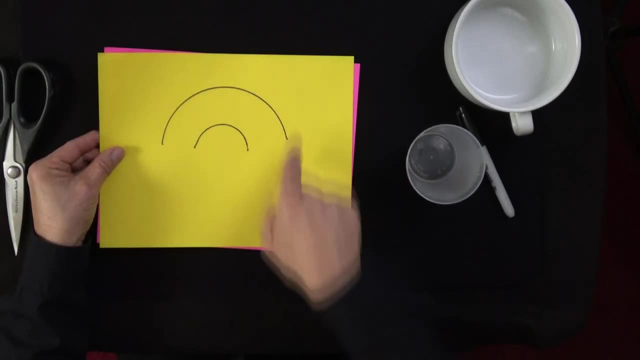 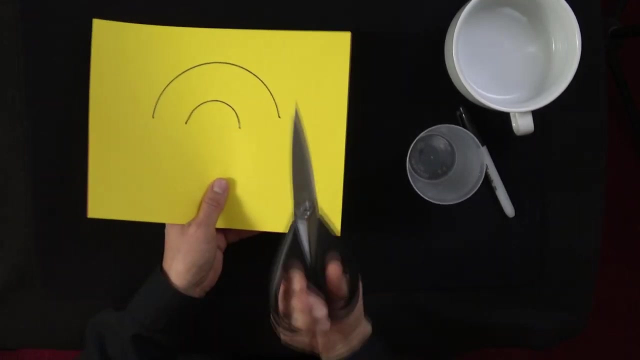 and that's looking pretty good. perhaps it's not as even as i would like, but that's okay. for purposes of the trick that will work. so we have an outer diameter semicircle, inner diameter semicircle, line the papers up, and now you're going to use your scissors to cut this out. you want the two papers together. 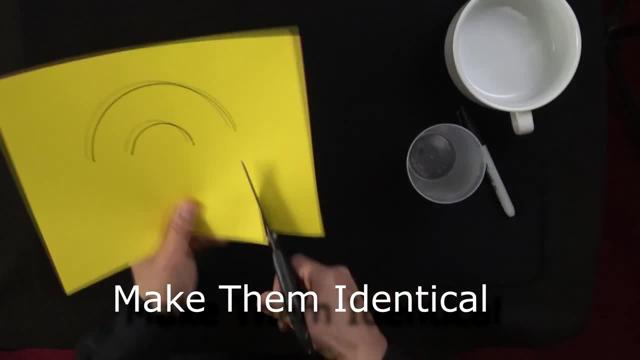 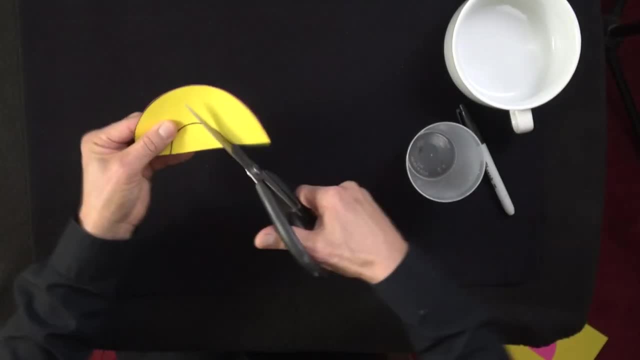 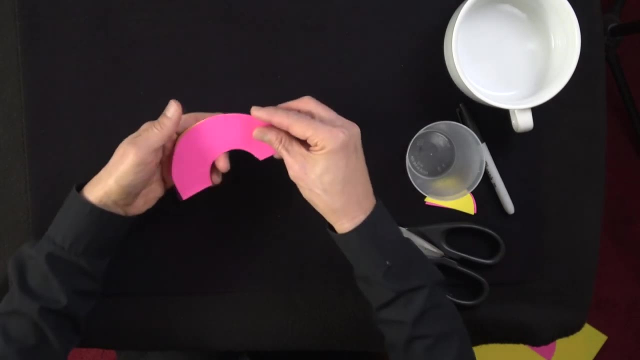 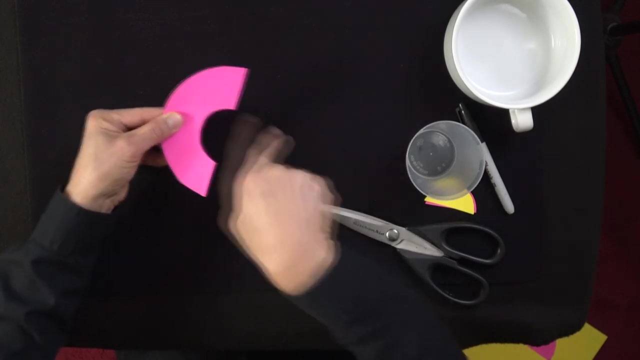 because you want these to be identical. so let's do that. now you have two arcs or rainbows, and the last thing you have to do is you're going to want to trim it somewhere about here so you don't have a semicircle. the trick works a lot better when you have 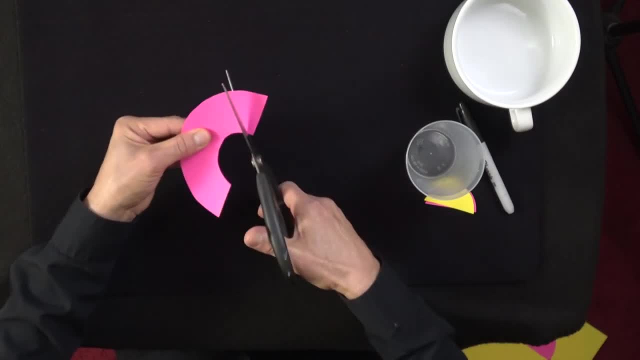 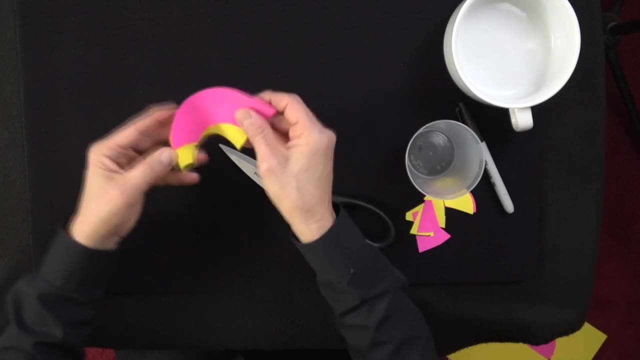 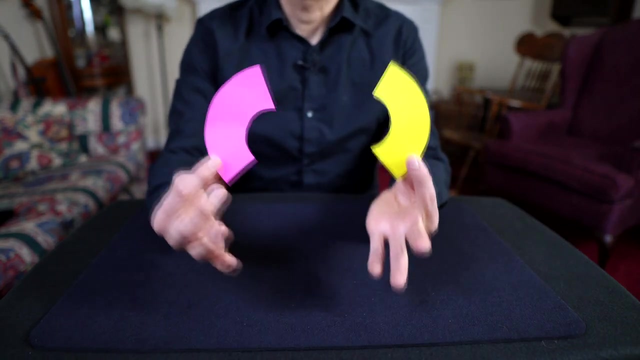 a shorter arc, so i'm just going to eyeball that in. i'm going to do something right about there and something right about there. now you have your boomerangs. here's how to perform the trick, as we showed you in the construction. the boomerangs are the exact same size. it's. 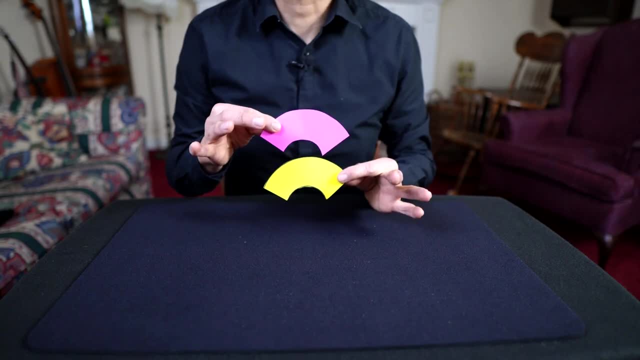 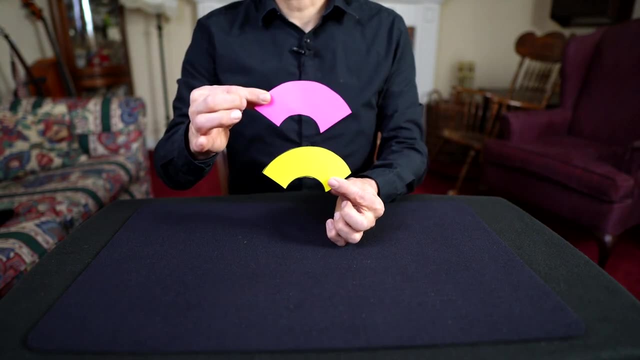 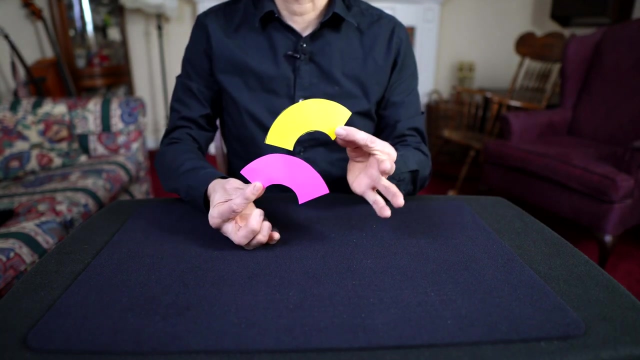 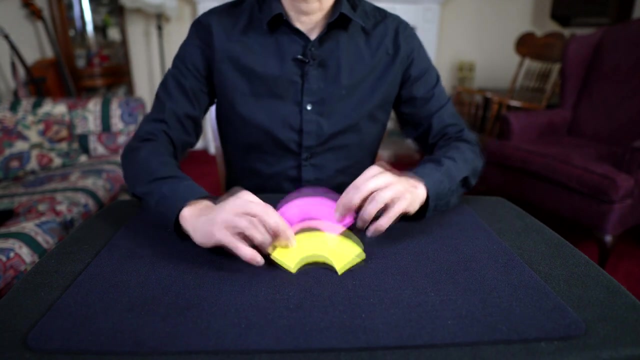 just an optical illusion. it turns out that whichever boomerang is held on top always looks smaller. so, no matter which way you hold them, the upper boomerang always looks smaller, and that's the secret. so all you have to do is just follow the storyline, just switch the positions and they'll change seemingly. 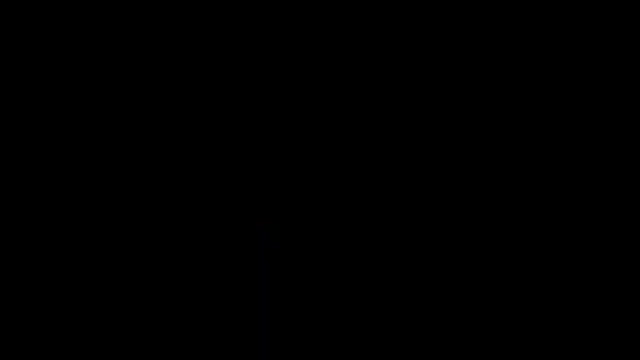 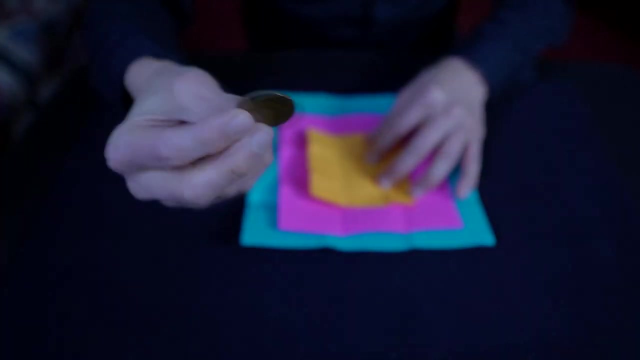 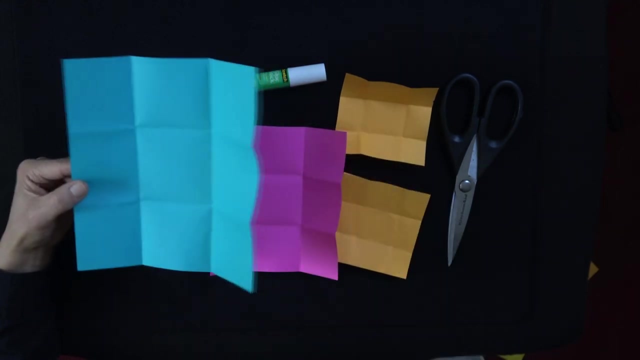 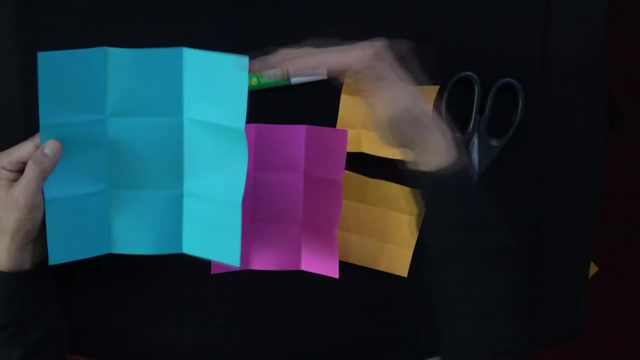 change in size for spectators. for this trick you're gonna need three sheets of paper, and what I'll do is I'll put the dimensions of everything up on the screen later on. but here I have a blue sheet of paper. what I've done is just taken a regular eight and a half by. 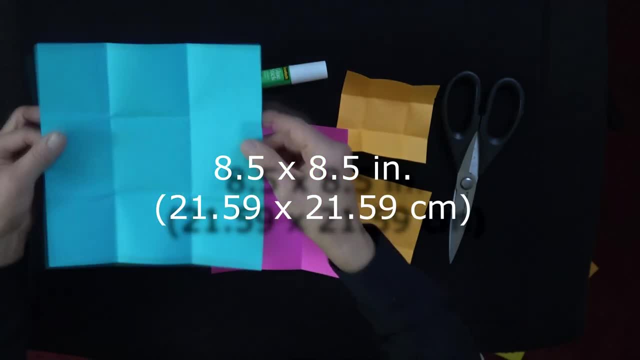 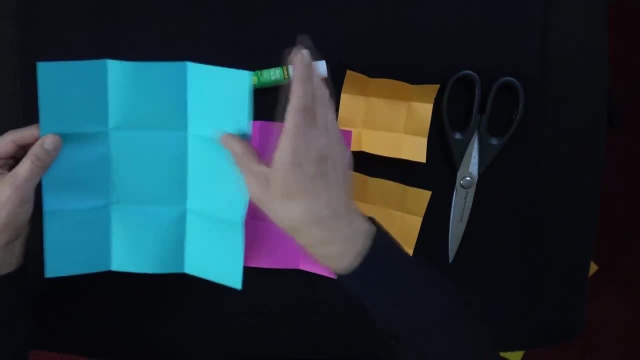 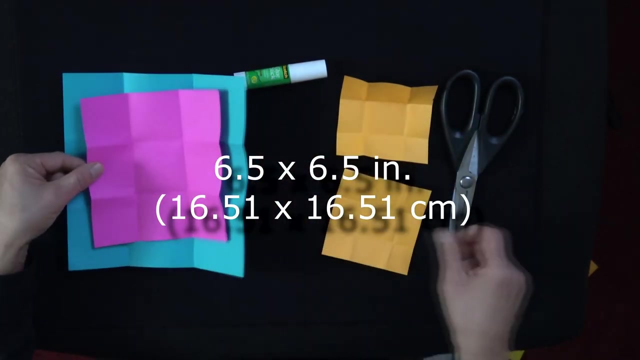 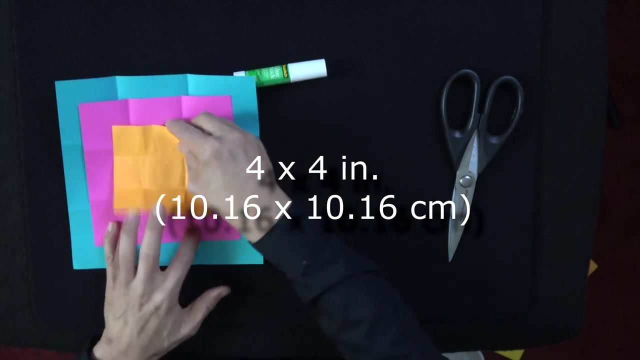 eleven sheet and lop this off, so it's a eight and a half by eight and a half square. just this is the normal distance on your standard printer paper. second, one is a little smaller and we have two smaller pieces that match, that are identical and are even smaller. so two of these are the key. 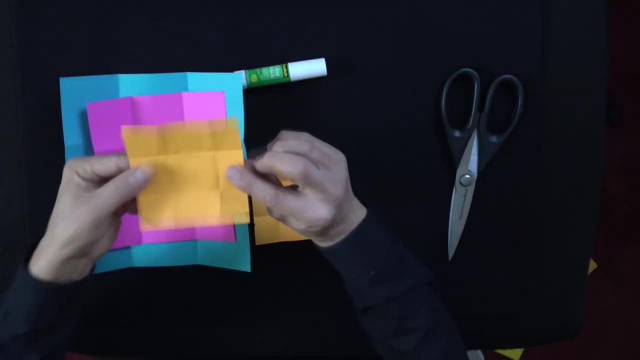 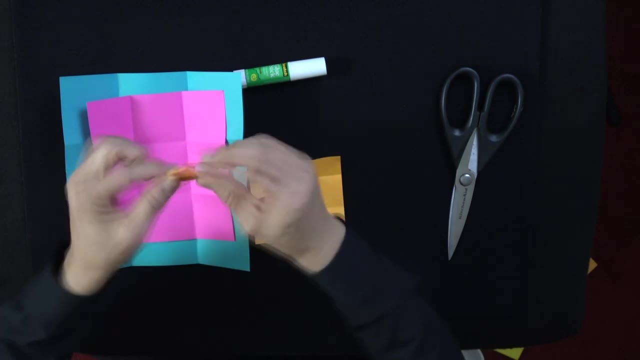 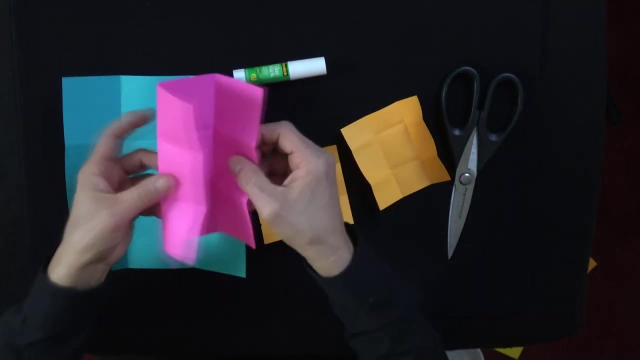 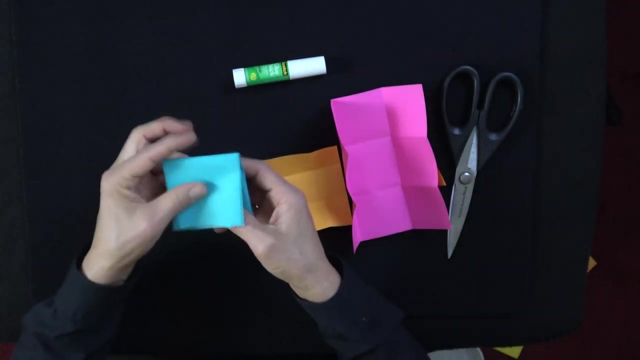 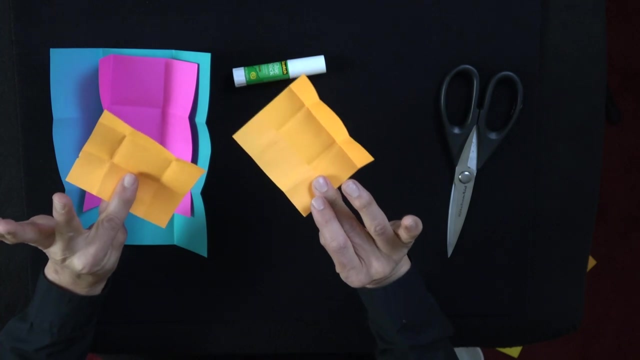 they have to be identical, and then what you do is take each sheet of paper and fold it in thirds, so you have something that approximates a square. that's done with all of the sheets of paper. here I've done that, and here I've done that. now the secret lies in these two pieces of paper you're. 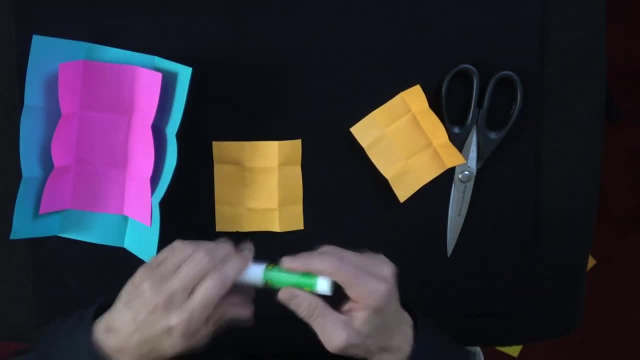 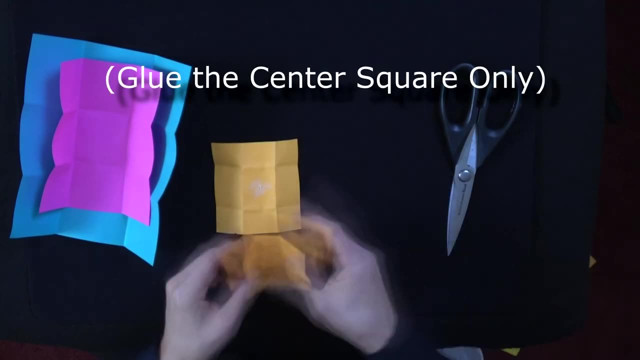 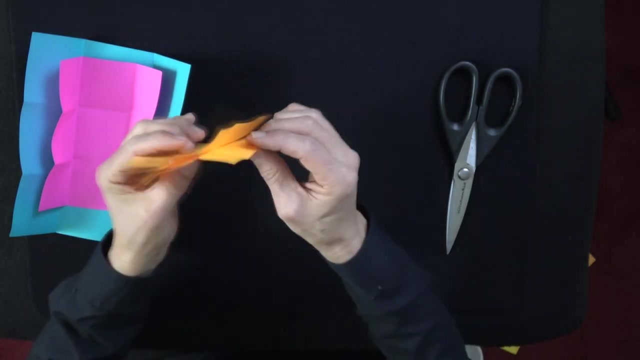 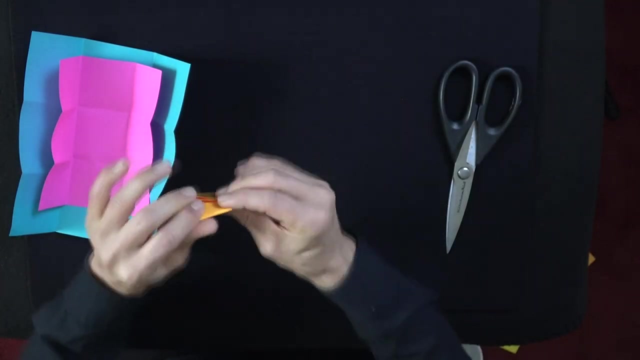 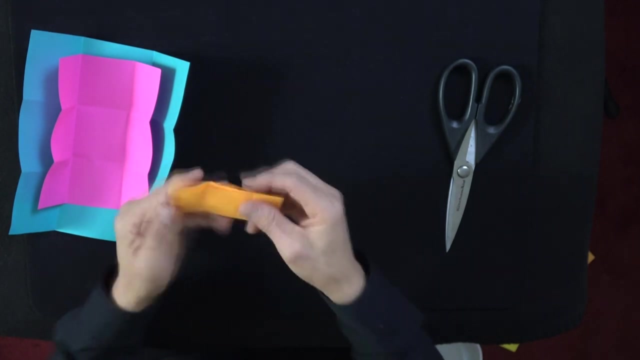 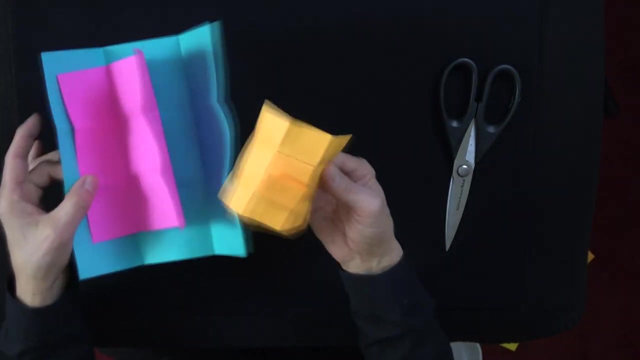 going to need some glue, and what you're going to do is take your glue and glue these two pieces back to back you. I'm going to use these two to fold in virtually the identical or same way, so you just create a single packet here, and therein lies the secret of the trick. so 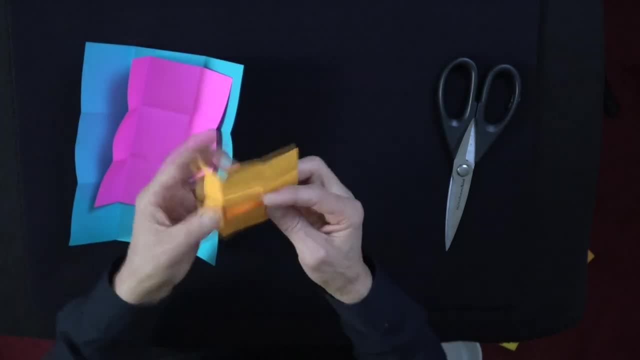 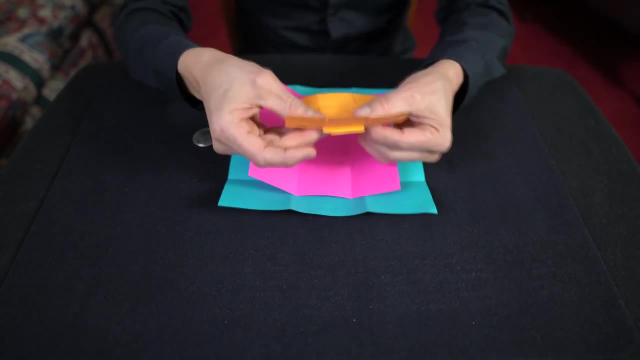 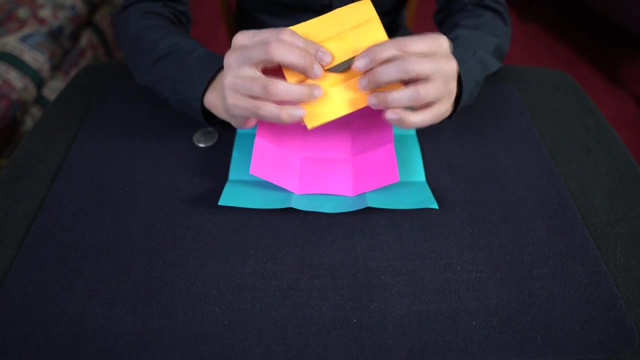 let's get into the performance and how to perform the trick. all right, I'm going to show you how to do the trick. I'm just going to do it in reverse. as you know from the construction, there's another side to this piece of paper, and so inside of here I have. 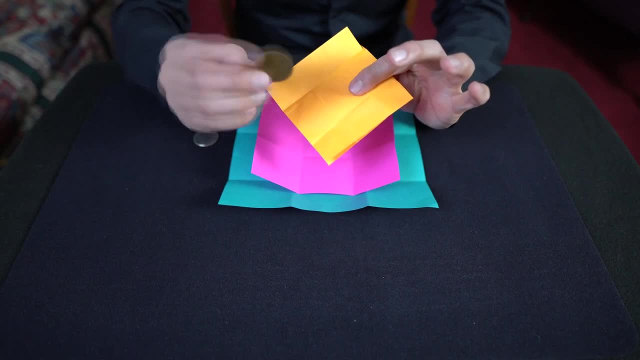 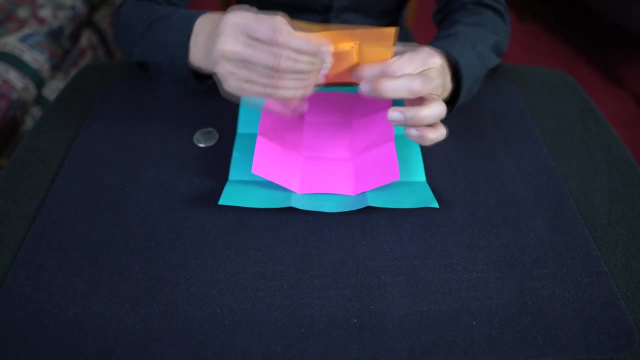 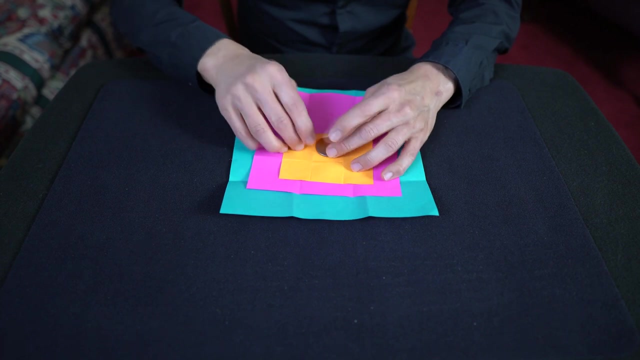 the different coin. so in this case we're just going to go backwards. I have the copper coin, the English penny, inside of here. fold it up nice and tidy, and I'm ready to start the trick. so I take my silver coin and I fold it in. now here's the sneaky part. 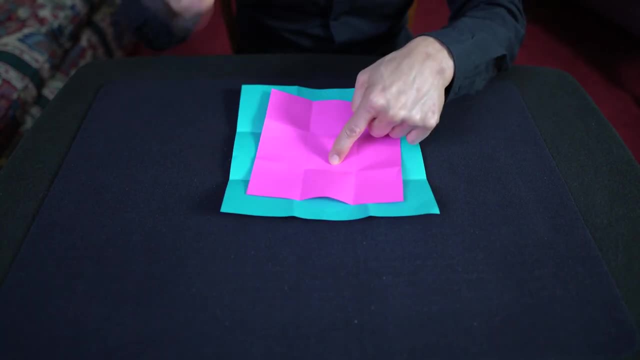 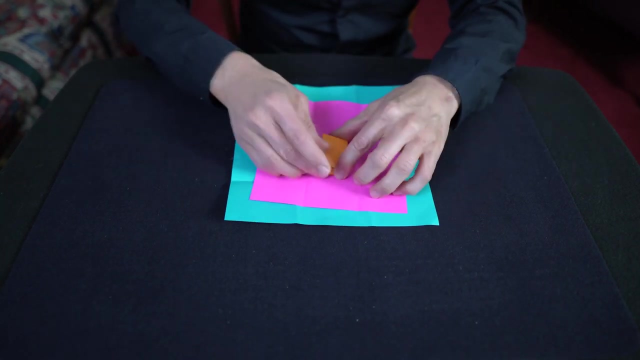 it's a little bit of misdirection, but when I say, look at this second piece of paper, I lift up this piece of paper here. but watch what I do when I put it back down. I've actually turned it over. let me show that to you again. so I lift this piece of paper, pointing out this piece of paper, and 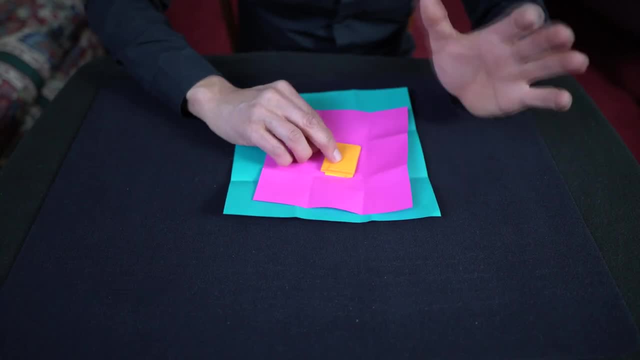 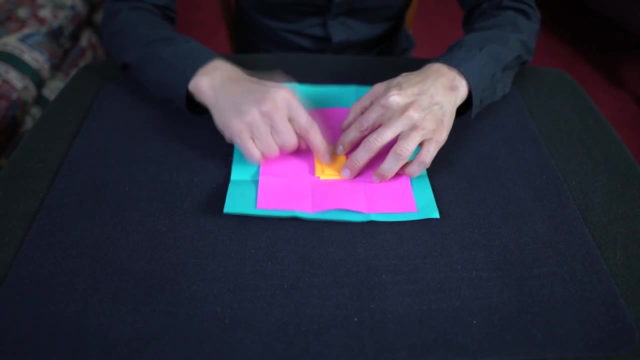 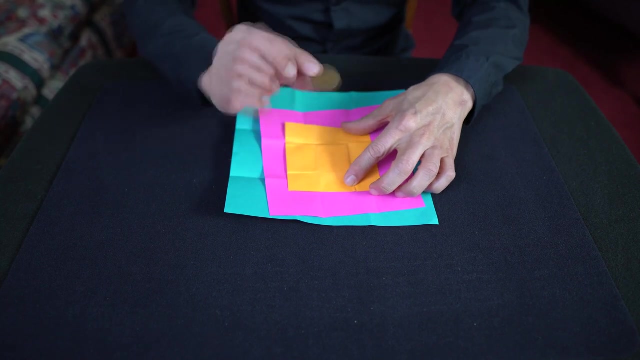 then when I put it down, I turn it over. a little bit of misdirection. they're pointing at the pink paper, but that's how I make the switch. so now the other side's on top, so now the coin will switch. so now, if I open this up, you'll notice that it's switched to the copper coin already. but of course, 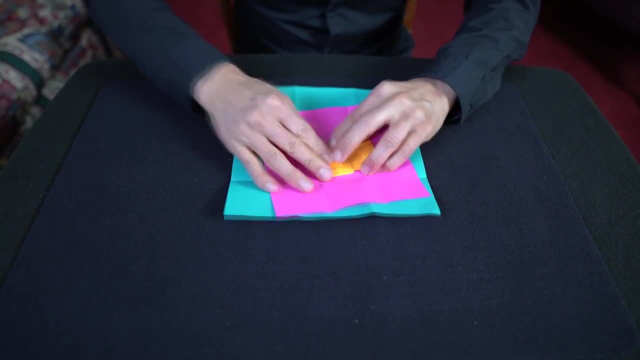 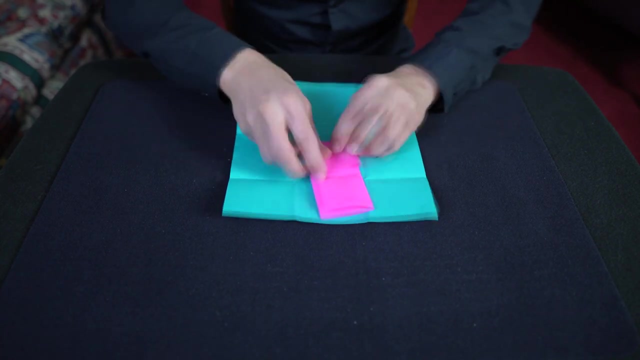 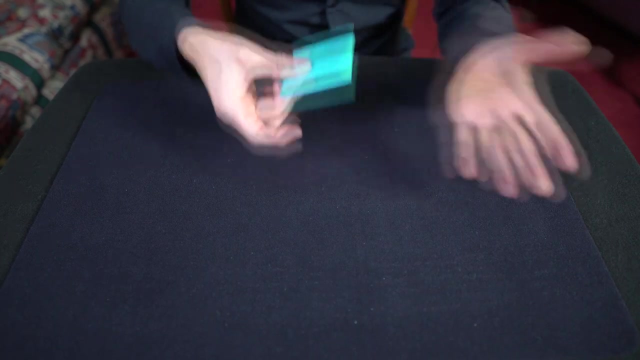 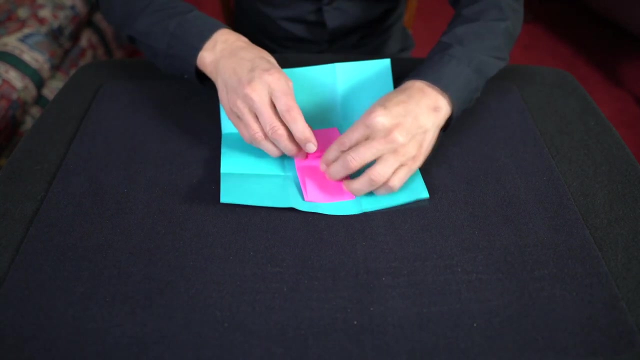 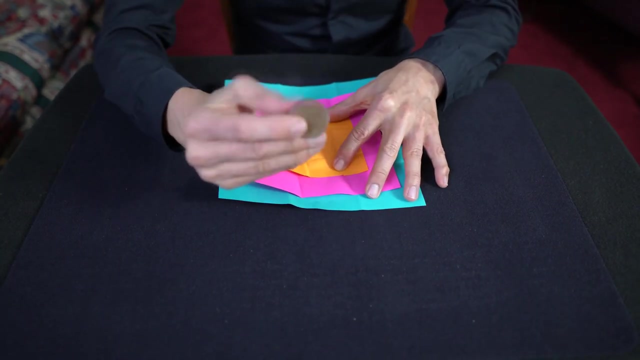 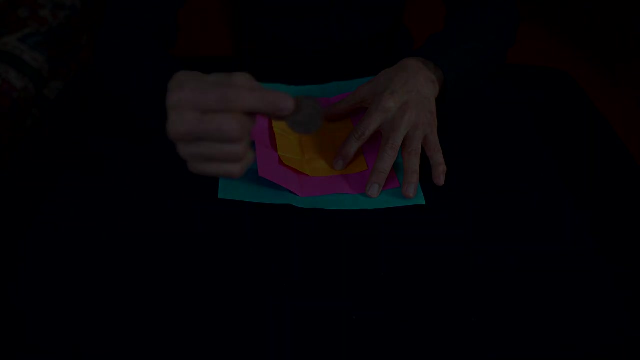 at this point, you've already done all the sneaky magic work, so all you have to do is fold up these pieces of paper. you can claim that you're just making everything as secure as possible. snap your finger and remember that coin that went in. open it up and it's changed into a copper coin. and that is the transformation of a coin. 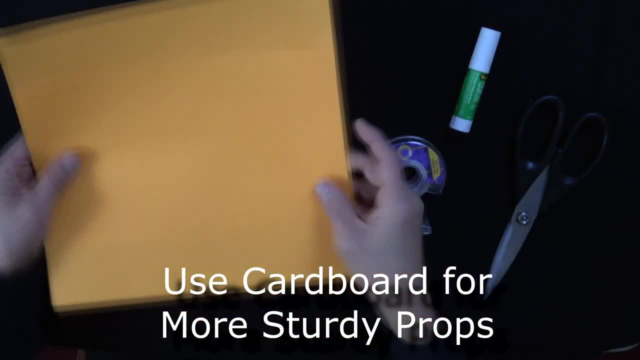 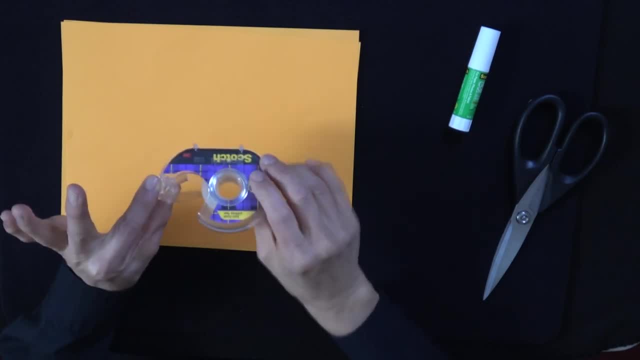 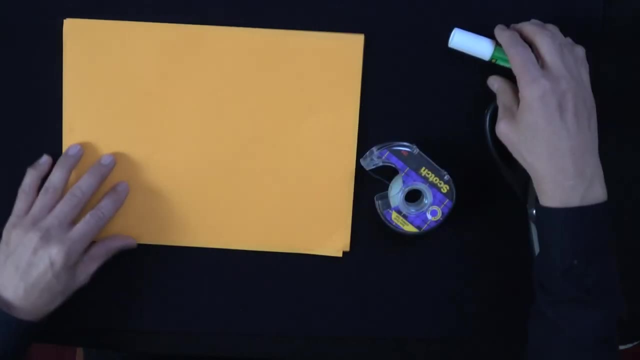 you'll need two sheets of paper the same color. of course, you can use white printer paper, it's just fine. you'll need some tape- actually, the tape is optional, but it really helps and I'll show you how, why it helps- and you'll need some glue as well as some scissors, so let's get. 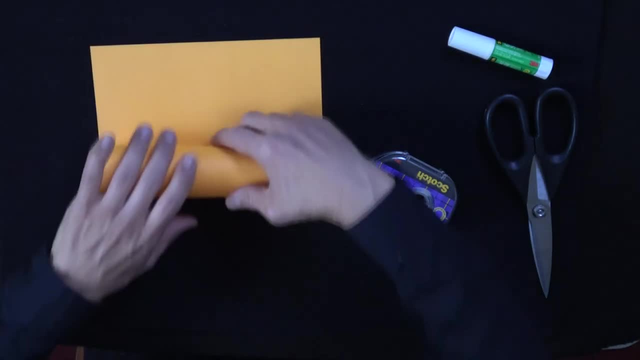 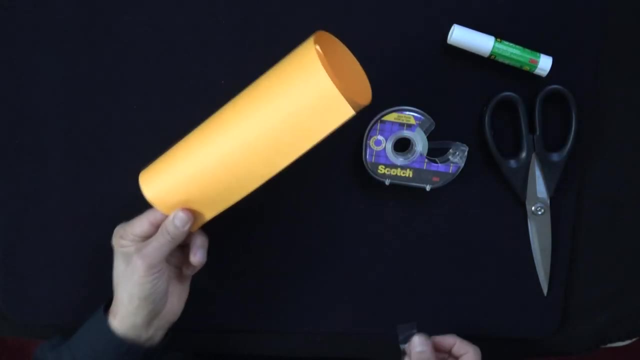 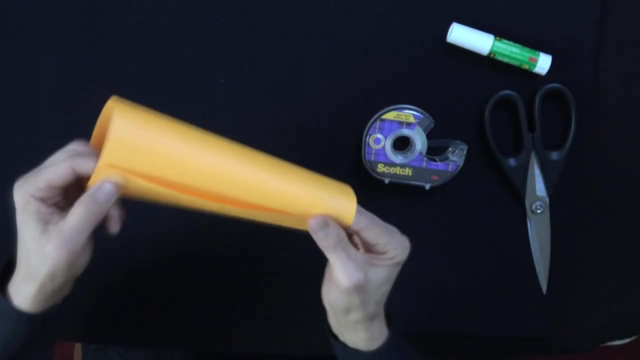 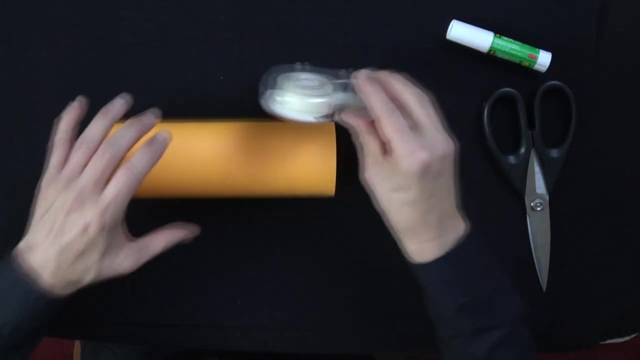 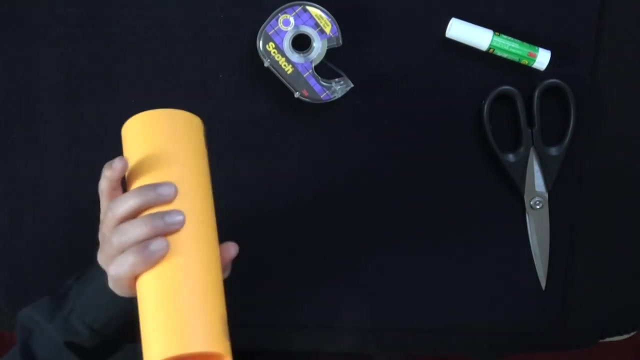 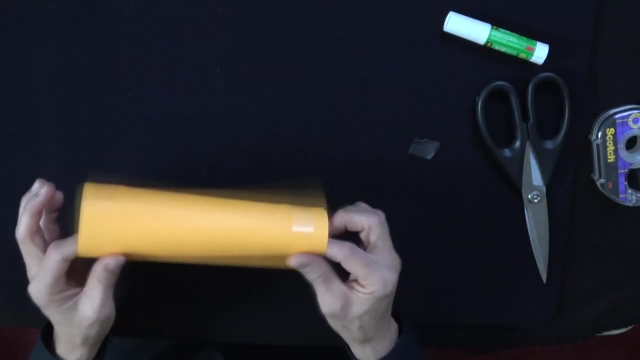 started. first of all, take your first sheet of paper and roll it into a cone, use a piece of tape and, just for good measure, I'm going to put a piece of tape along this seam here and now I have a fairly nice clean tube. second sheet of paper. now this part gets a little tricky. 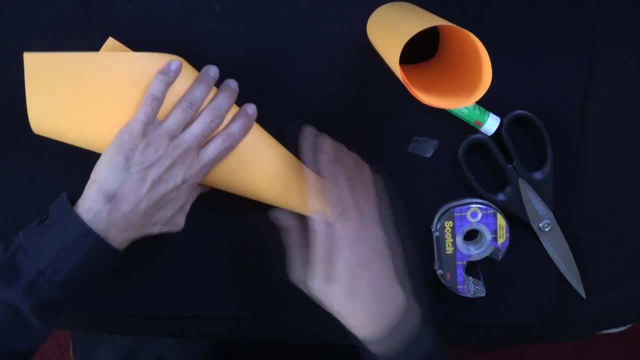 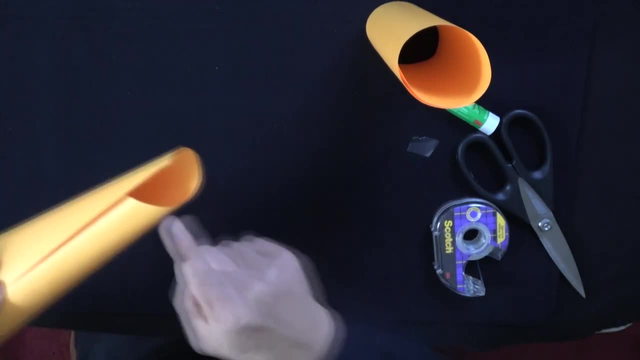 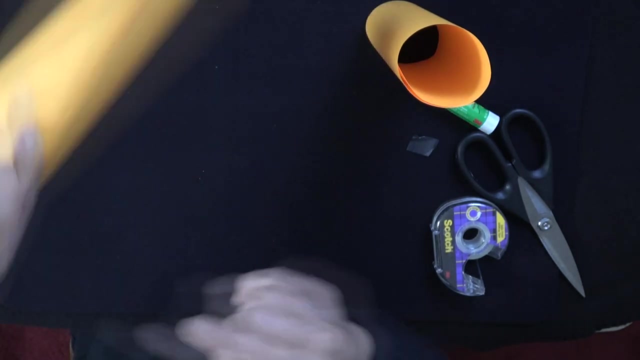 what you're going to do is make something of a cone, but it's not actually a cone. it's going to want a rather small opening here. you might have to experiment a bit, and you're going to want to keep it fairly wide. at the other end, you're just making a another cylinder. 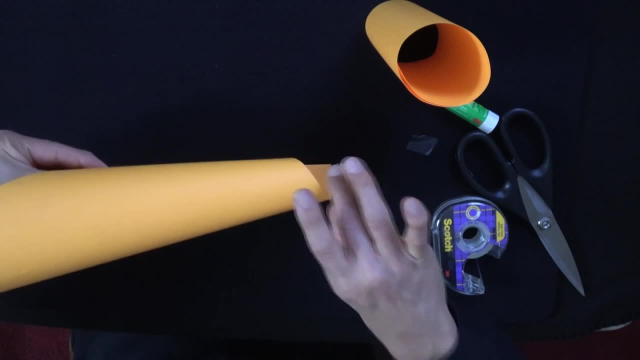 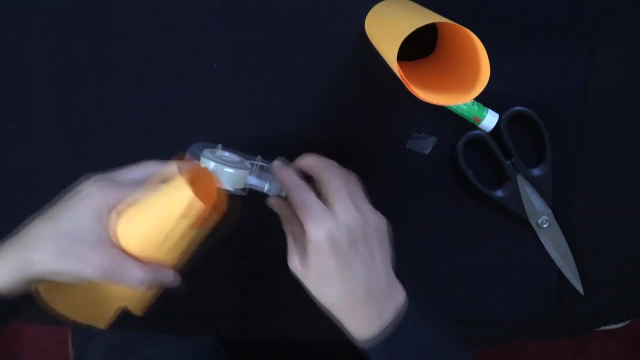 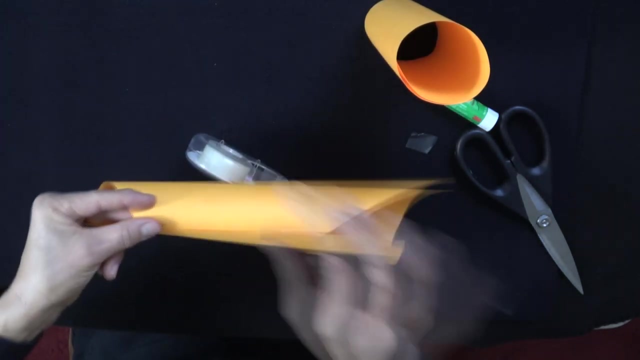 but it's lopsided. one side is wider than the other. take a piece of tape and hold it there. helps to have two pieces of tape on it here, because this, admittedly, is a little awkward. While this trick is great for little kids to perform, it's not an easy one for the kids to put together, so an 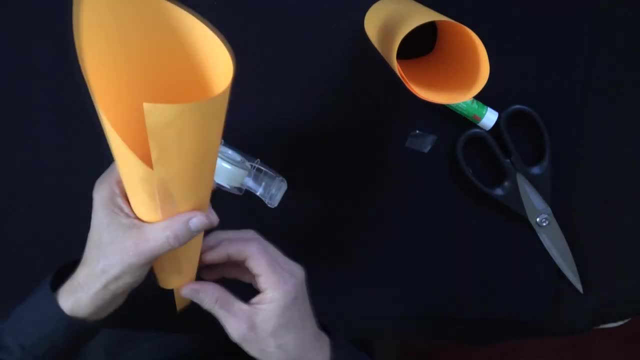 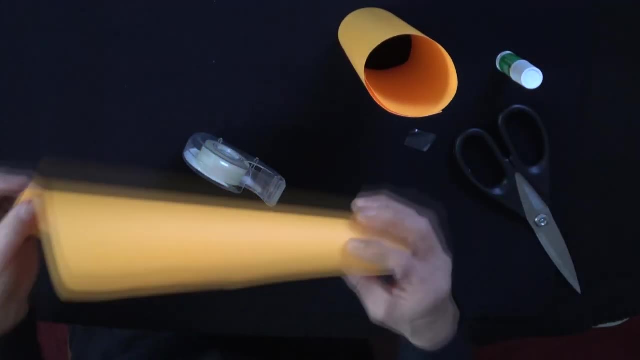 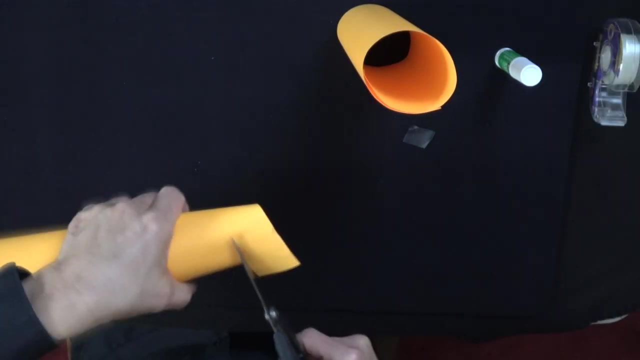 adult might need to put this one together for the youngsters. We have our regular cylinder over here and we have here a lopsided cylinder. What you're going to do is cut a line right here, so you want to straighten this out? Now take your. 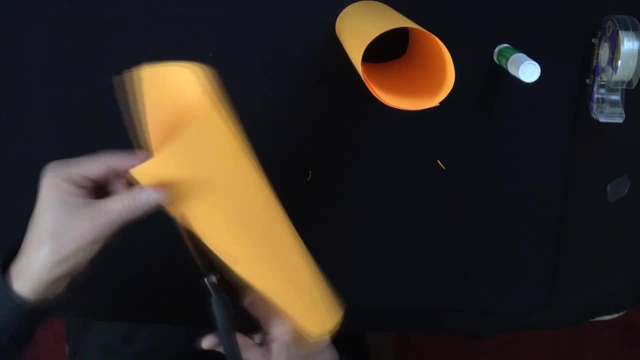 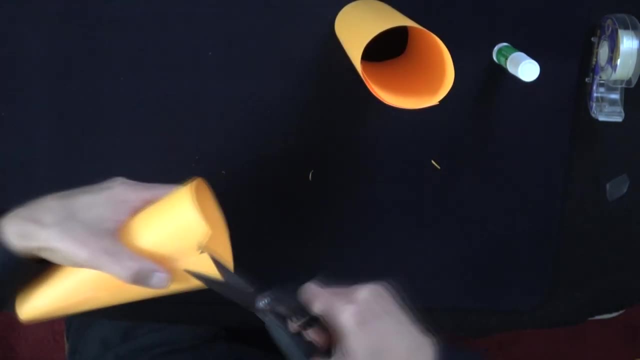 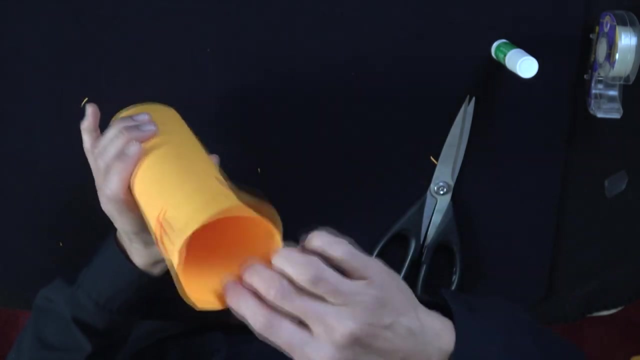 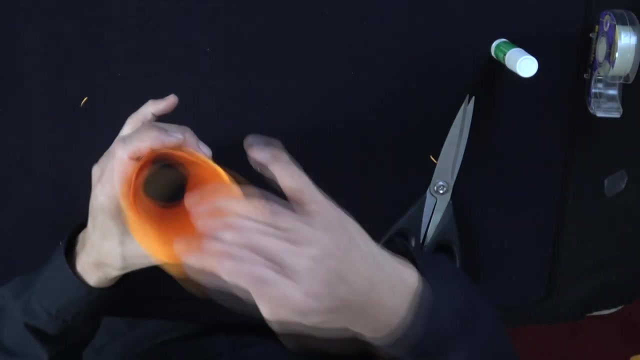 scissors and do the same thing. over here I now have a cylinder that's slightly lopsided. Take this lopsided one and you insert it into the other cone Or cylinder there. That's looking pretty good. so what I'm going to do now is I'm 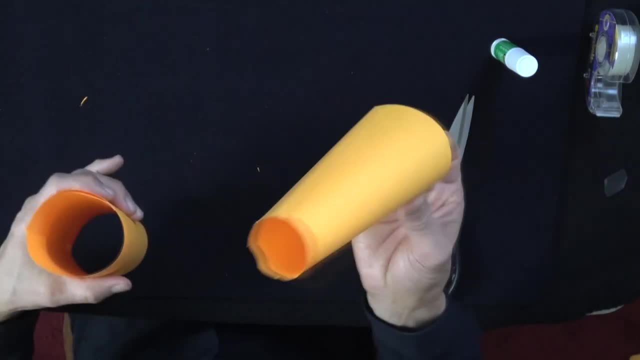 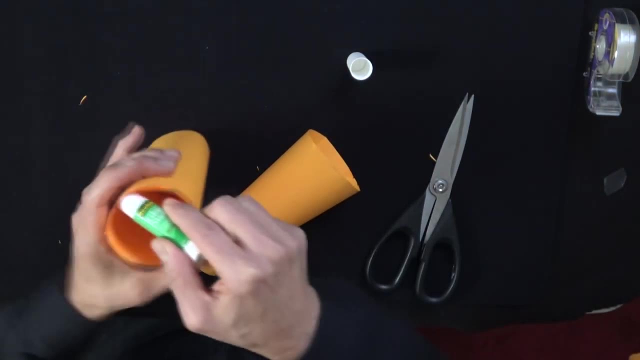 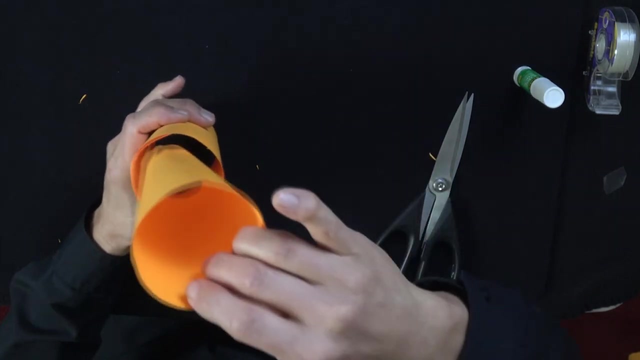 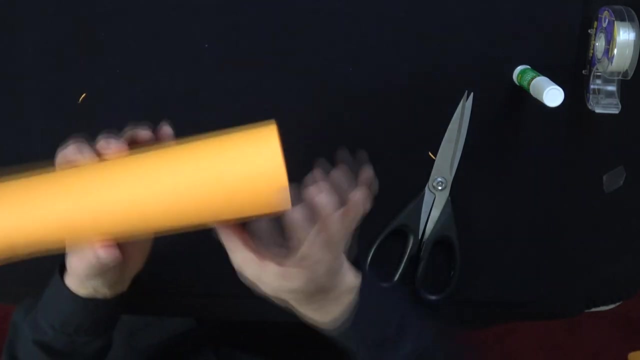 going to put some glue on the inside of here so that will take and hold this right inside here. Now take your cone, place it inside so you're adhering this cone to the other, the other cylinder. but if you look from this direction, you'll see that there's this cone here inside and 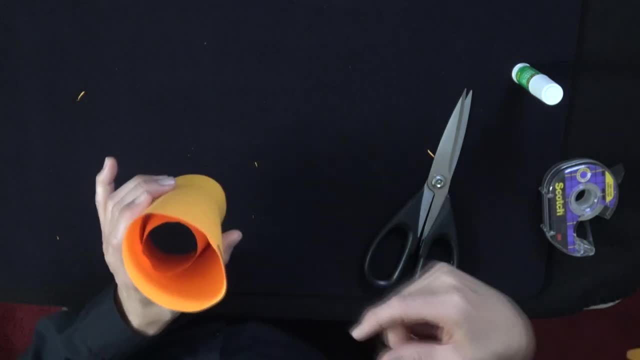 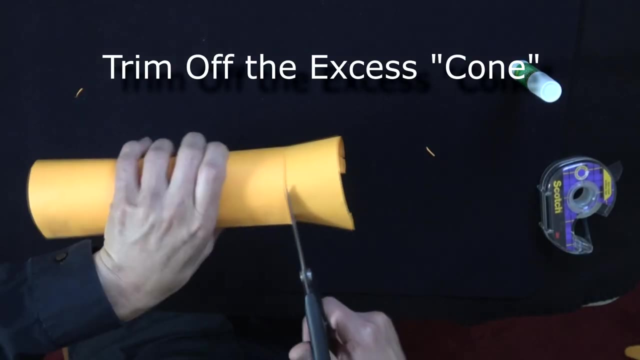 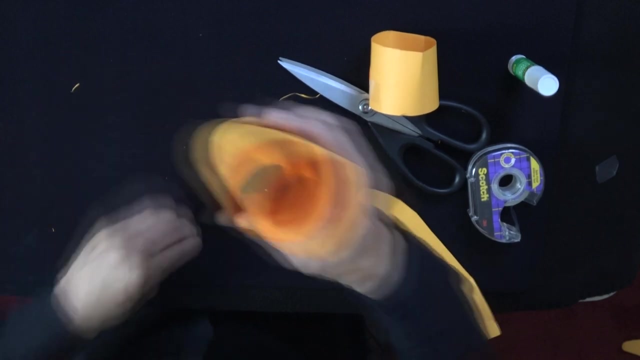 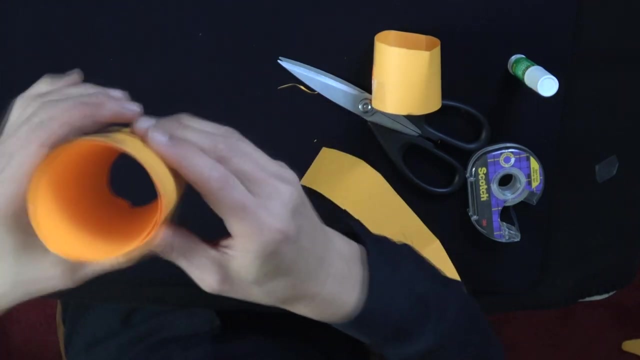 There's actually room on the sides to put things over. on this side It looks fairly normal And there now it's ready to perform the trick. as you can see From this end looks fairly normal. something I would Recommend is if you have some different colored tape. 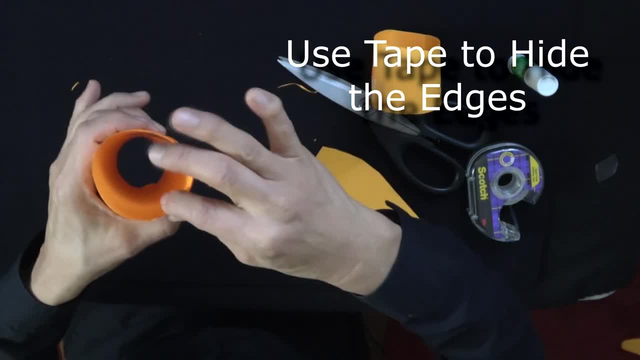 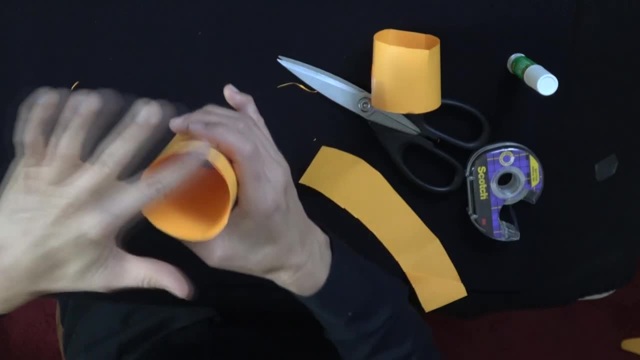 Color tape here, like maybe in a red or green or something. You can put it along this edge and kind of seal it up. if you do this close up to people, They might notice that there's a slightly Slightly ragged edge here, so you can show the tube. 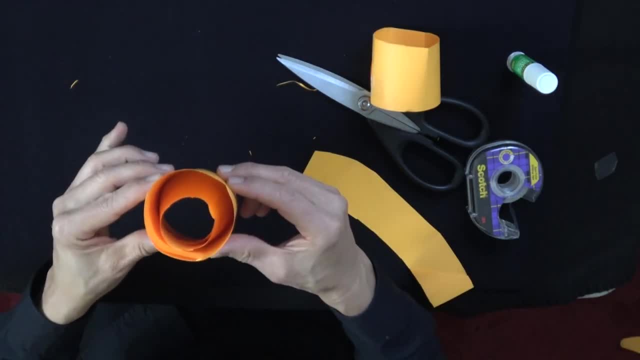 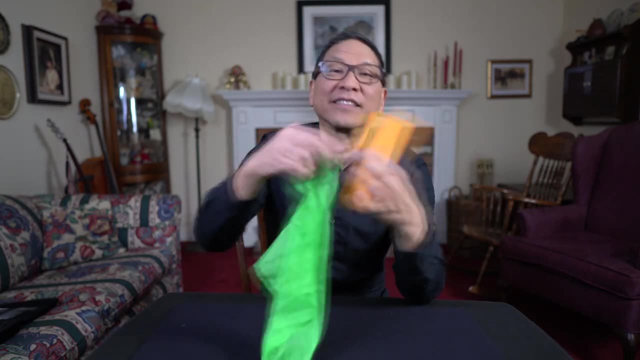 empty and Still have room to hide things. And let's get into this Explanation of the trick. now you've made your tube, you're ready to set up for your trick. I've been to be using a handkerchief here, very thin silk handkerchief. 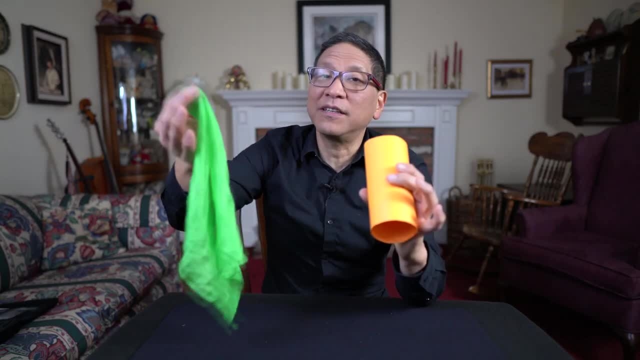 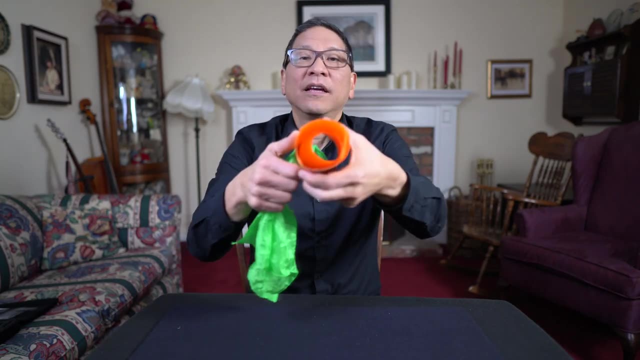 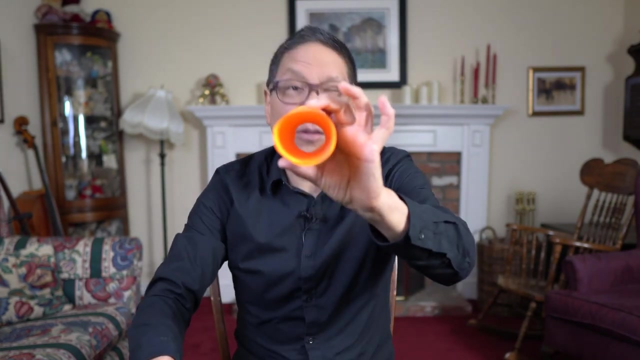 You can use confetti, you can use ribbons, whatever you can fit inside of the tube. so, beforehand, I think you already know the secret from what we've taught you. but, as you know, there is a secret compartment inside of here and by using that little conical piece inside of the other one, it creates a 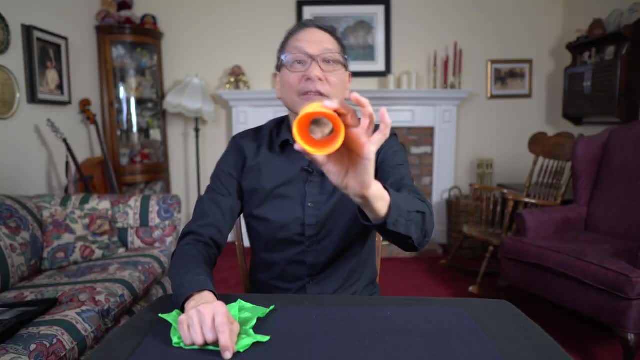 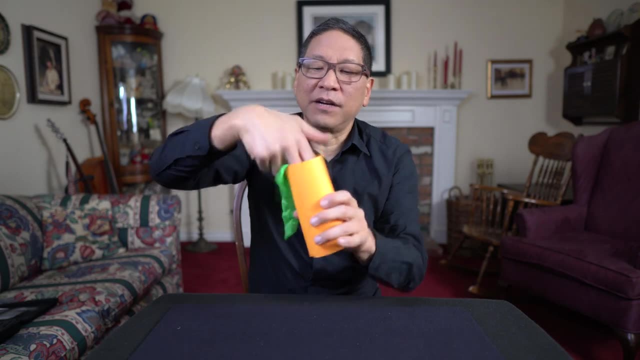 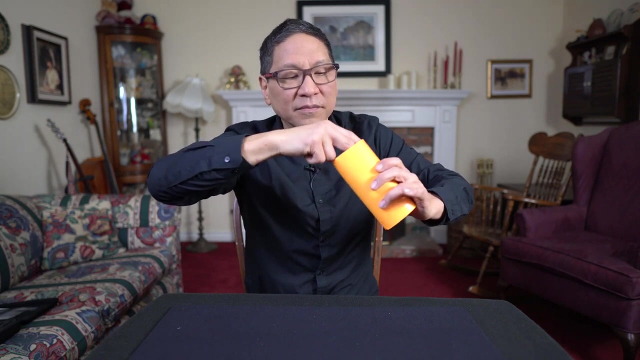 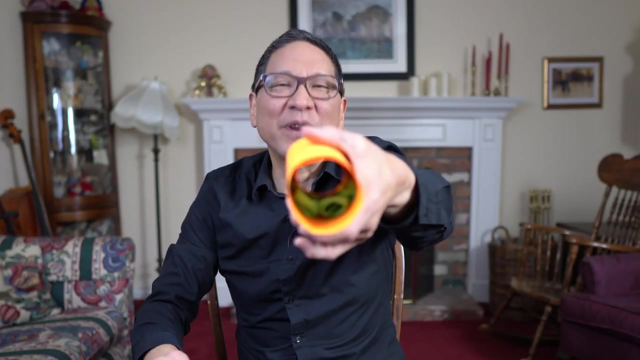 Forced perspective. that's what it's called, and it looks like the tube is normal. However, it is not. beforehand, take your ribbons, confetti, Whatever it is. you're just going to place it Into the tube Along the side, right there. Now you're ready to begin the trick. 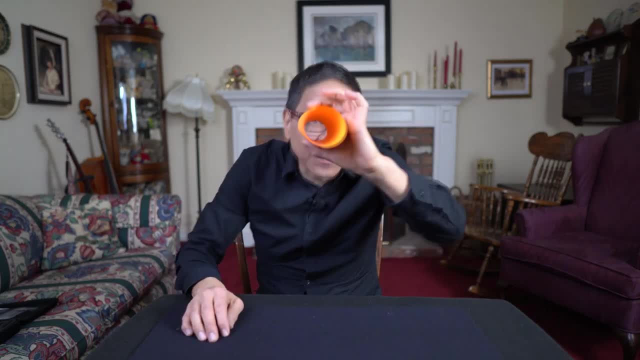 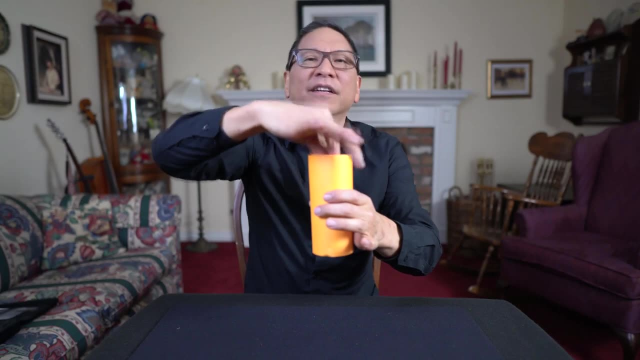 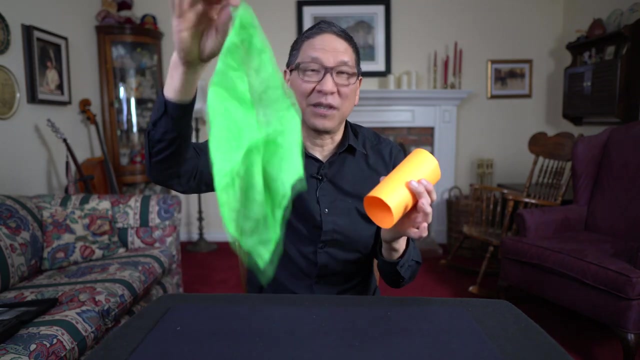 You just walk out, you show you have a tube and you can even do this, so people can see that the tube is empty. and then all you do is snap your finger, reach in and produce your handkerchief, your confetti, whatever it is that you want to bring out. 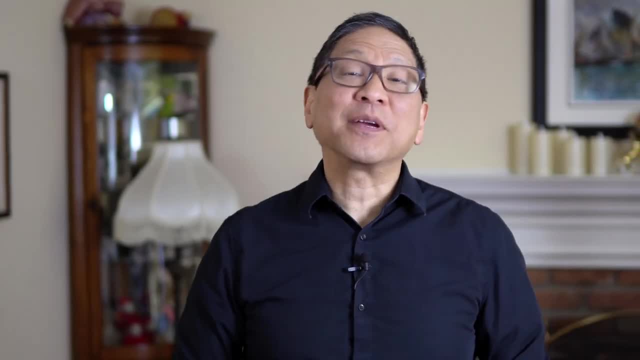 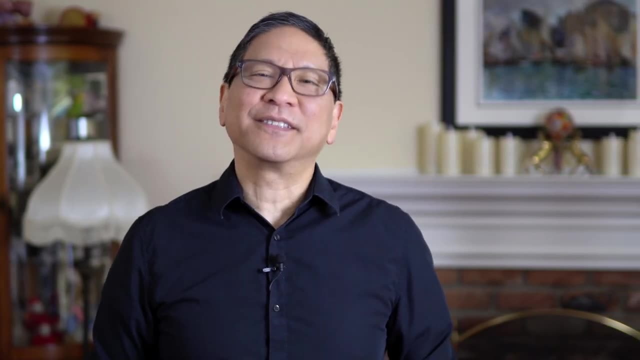 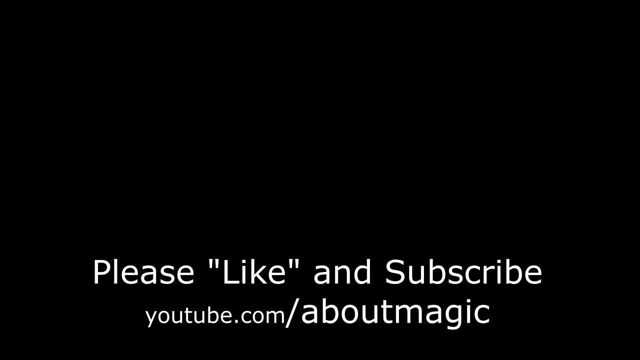 well, i hope the kids in your life are having a blast performing these magic tricks for friends and family. please give us a like and please subscribe for more magic lessons in the future. thank you for watching. i'll see you next time you.